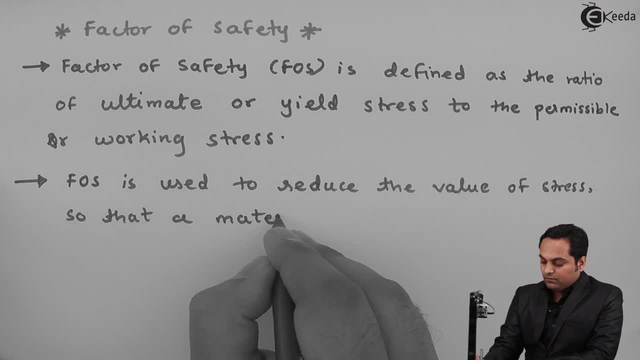 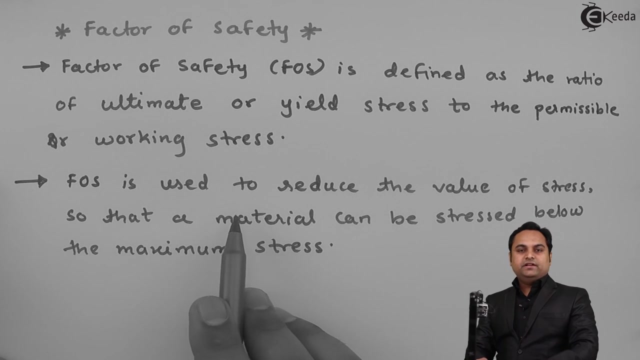 or material stress to the permissible or the material stress Dit. here it is stressed- below the maximum stress. We can also use this Теперь statue factor of safety. At the end of the study it is used to reduce the value of material stress. 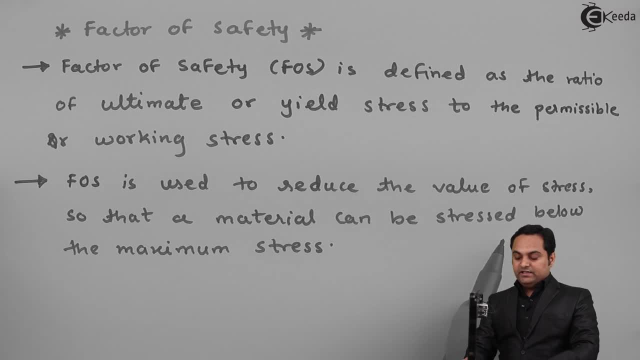 So that the material can be stressed below the max value. This st slowing in this 돈 family Because we don't want the material st slowing down. It is not st slowing down to operate in the maximum stress region, because if the material reaches maximum stress after. 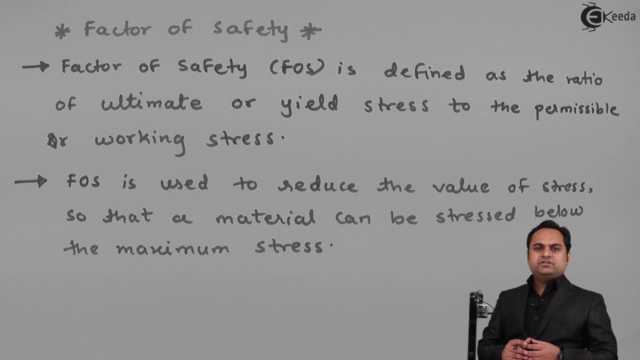 that even if we reduce the value of stress then the material would be failing at any low value of stress. so to avoid the failure of material it is necessary that the material operates below maximum stress. so we divide the value of the stress by a factor, and that is called as factor of. 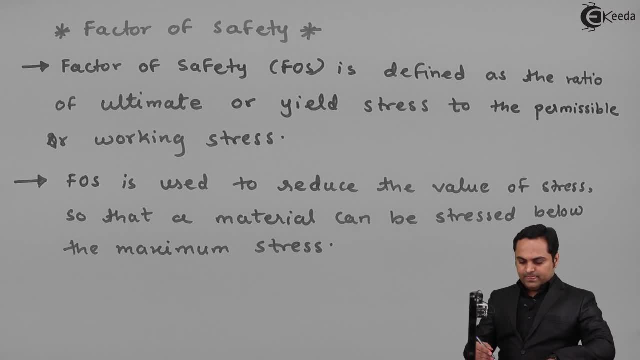 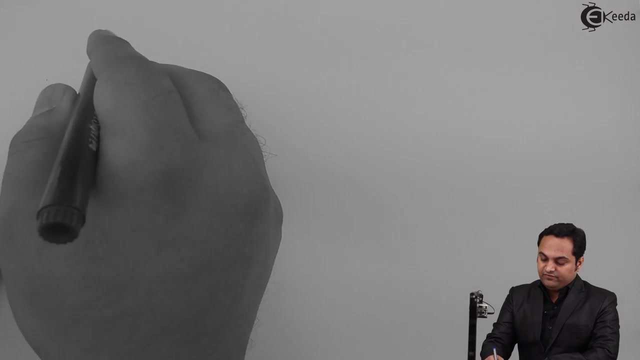 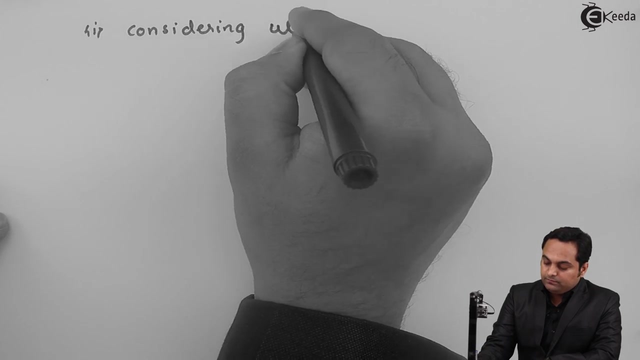 safety to get the permissible or working stress. next, FOS is always greater than 1. next, FOS is a number and it does not have a unit. so after this I can write the formula of FOS. so first I'll write down, considering ultimate stress. so 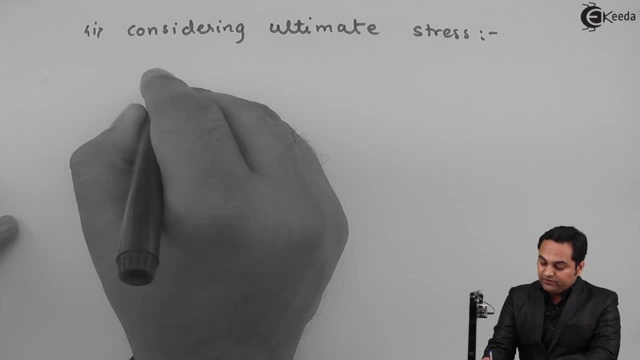 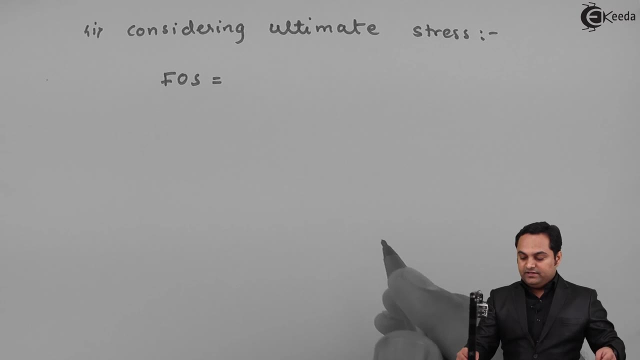 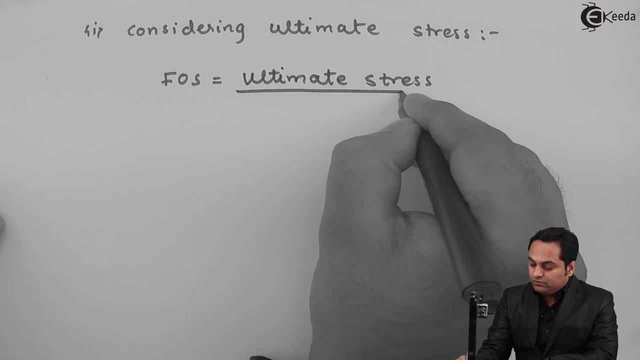 when we are using the ultimate stress. so factor of safety as it is defined as the ratio of- I have written here for rest of a factor, wait here while this process is separated. so the this is the duration of continuous test, and Sell cost will be given as the. 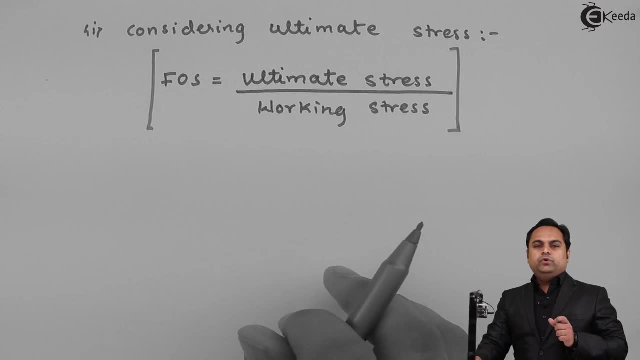 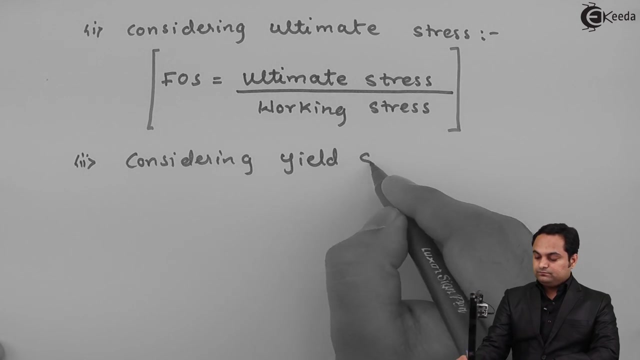 maximum stress, just like the total stress in which the material becomes 내�ent. so when the material achieves its maximum stress, the value and appearance of the material is allowed in FOS. Next, considering yield stress. factor of safety is given by yield stress upon working stress.